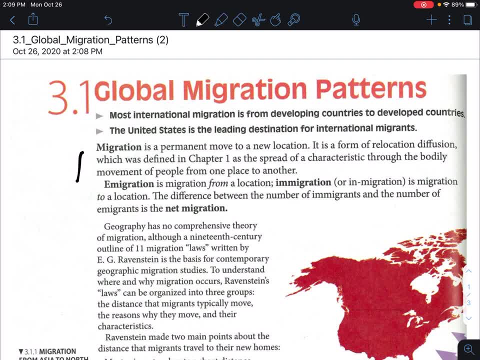 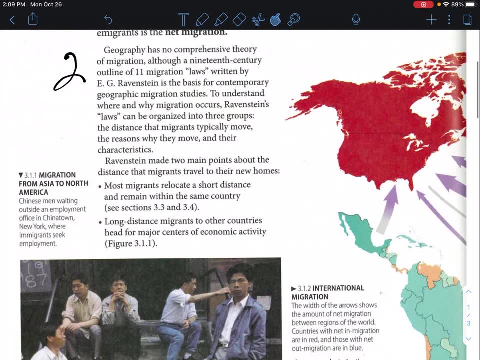 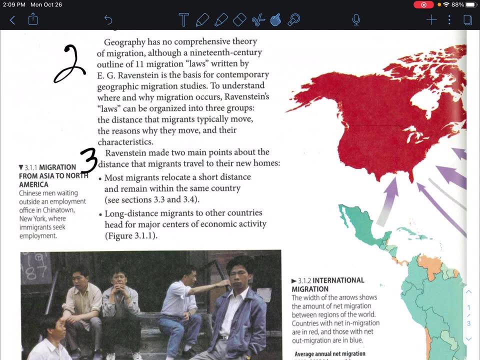 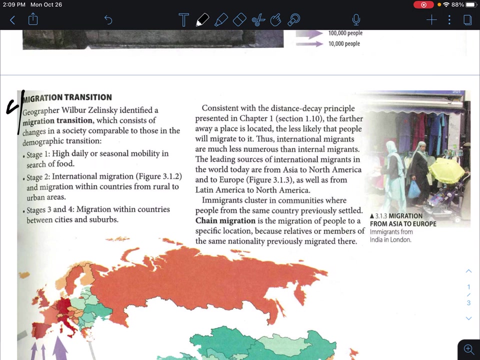 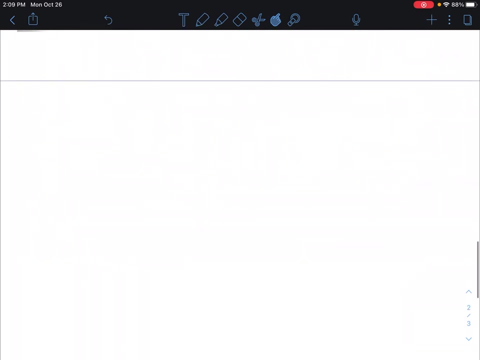 paragraph number one. I am going to number paragraph number two. I am going to list this one as paragraph number three And I am going to include those bullet points in paragraph number three. I am going to label paragraph number four, five, six and I believe that is all our reading has. So six paragraphs, not a whole lot. I'm 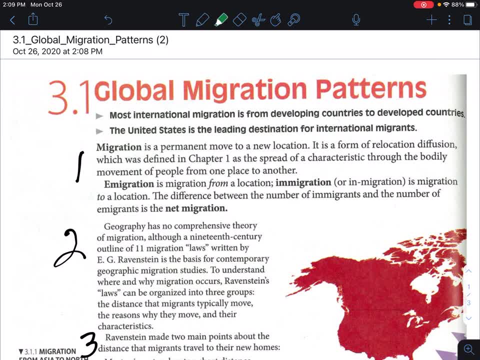 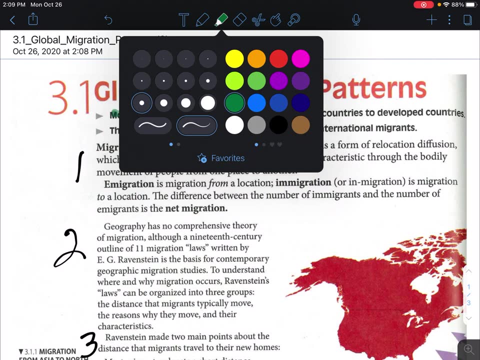 going to grab my highlighter now and start marking my text. Global Migration patterns. Most international migration is developing is from developing countries to developed countries. So I'm just gonna go ahead and whoops, I'm not gonna highlight that. I'm gonna highlight with something a little bit brighter and I'm 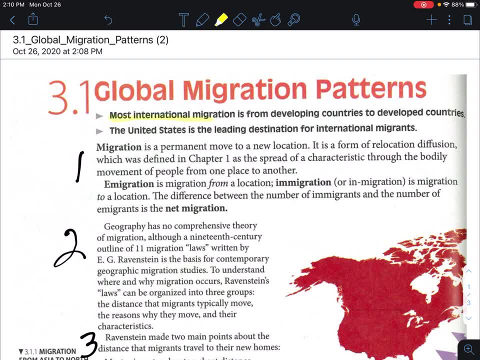 going to undo that and undo that. Most international migration is from developing countries to developed countries. The United States is the leading destination for international migrants. Migration is a permanent move to a new location. It is a form of relocation diffusion which was defined. 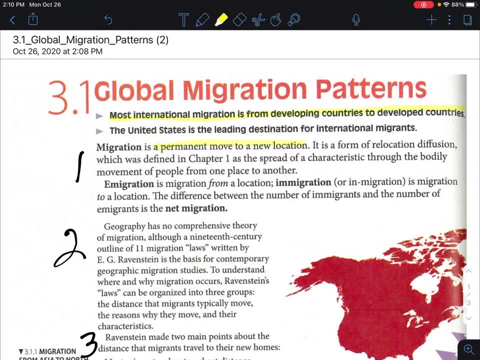 in Chapter 1 as the spread of a characteristic through the bodily movement from one place to another. So one thing I'm going to do here is just circle the key term of relocation diffusion. So one thing I'm going to do here is just circle the key term of relocation diffusion. 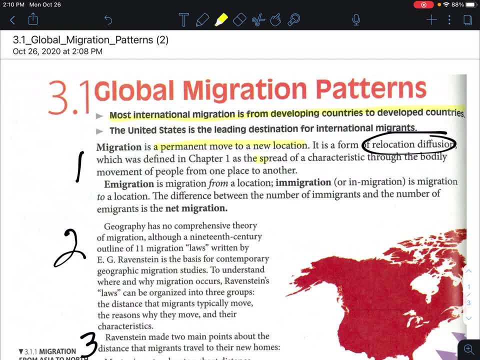 And then we're going to highlight its definition: the spread of a characteristic through the bodily movement of people from one place to another, to another. Bodily movement literally means a person is their physical body is moving from one place to the next. Immigration, migration from a. 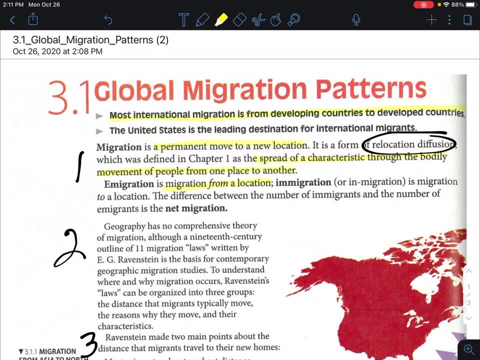 location with the letter E. Immigration or in-migration is migration to a location. We've got another definition right in here. The difference between the number of immigrants and the number of immigrants is net migration. I'm going to undo that last one. So there are a few things going on here. 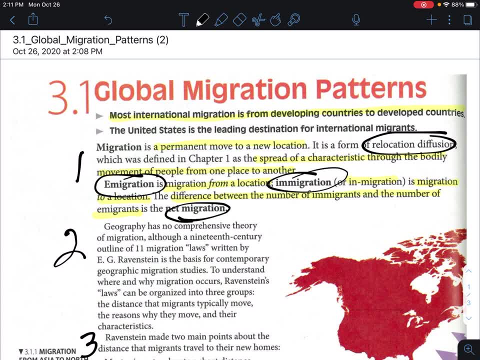 I've got definitions for net migration, immigration and immigration. It's tricky that they sound exactly the same although they are spelled differently. There is a term for that in the English language. Spelled differently sound the same is an homophone. A homophone is a word that. 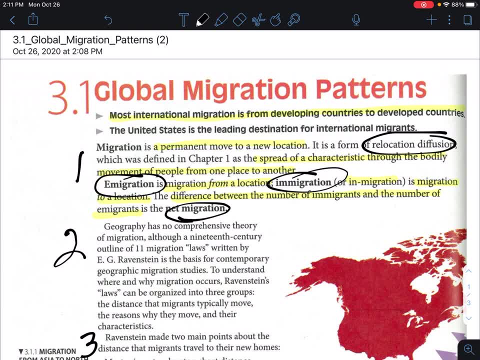 sounds the same as another word but has a different meaning or spelling. So there's immigration with an E and for that one I'm just going to put in a little note here: Immigration with an E. I always think of the E as exit and I left that place. Immigration with 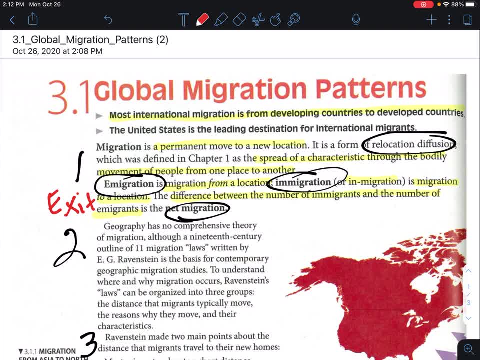 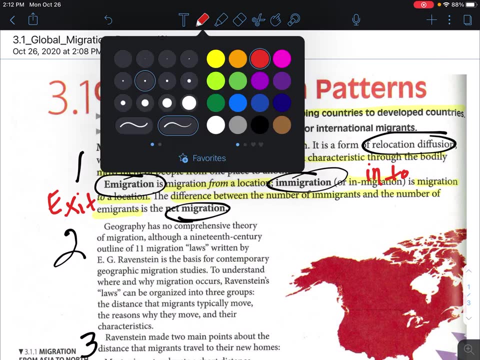 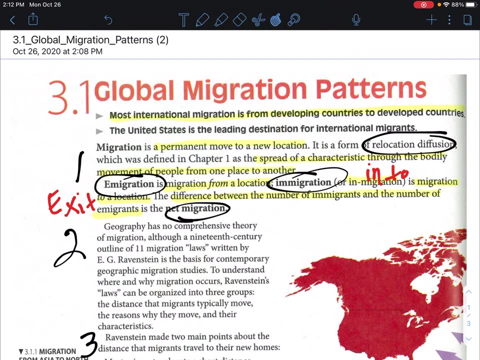 the I. I like their definition right here or their example right here: The I in immigration, meaning like to go in to a new place. So that's just what I use in to make it helpful for me to distinguish between those two words, those homophones that sound the. 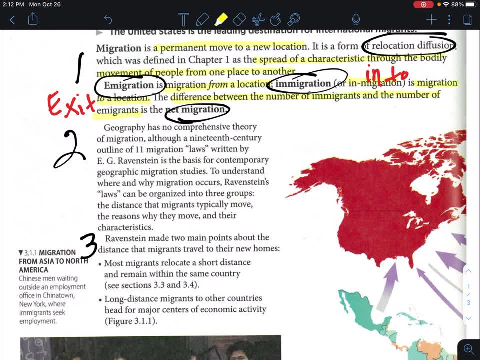 same but have a different meaning. I'm going to go back to my highlighter. read paragraph number two. Geography has no comprehensive or complete theory of migration, although a 19th century outline of 11 migration laws written by EG Robinstein is the basis for contemporary geographic migration. 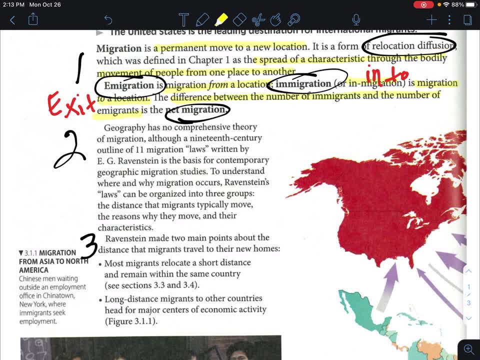 studies and you read about Robinstein's laws for migration in the chunk portion of today's lesson. To understand where and why migration occurs, Robinstein's laws can be organized into three groups: The distance that migrants typically move, the reasons why they move and their characteristics. Robinstein made two points. 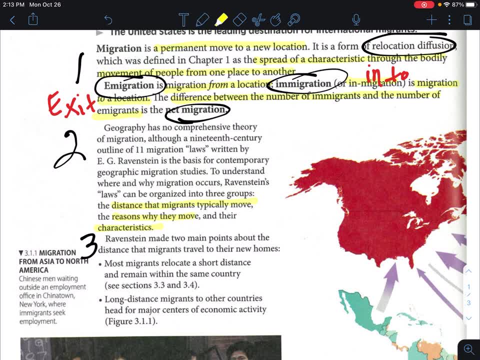 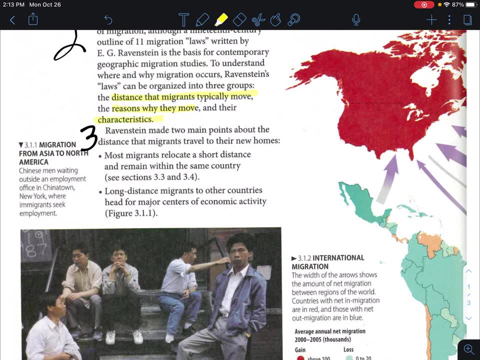 about the distance that migrants travel to their new homes. Most migrants relocate a short distance and remain within the same country. Long-distance migrants to other countries head for major centers of economic activity- And what's another way to say economic activity? They are looking for jobs. 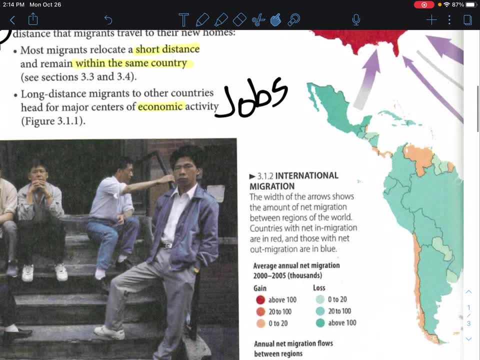 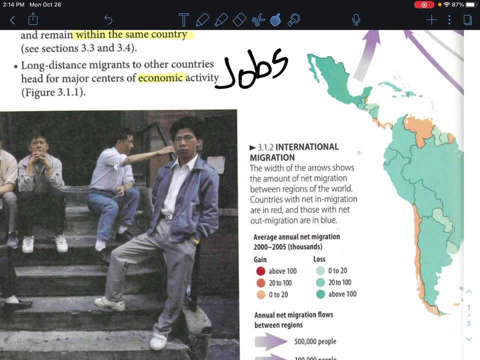 We have an image here I'd like to share with you: international migration. The width of the arrow shows the amount of net migration between regions of the world. Countries with net in migration people are moving in are in red. They're gaining. 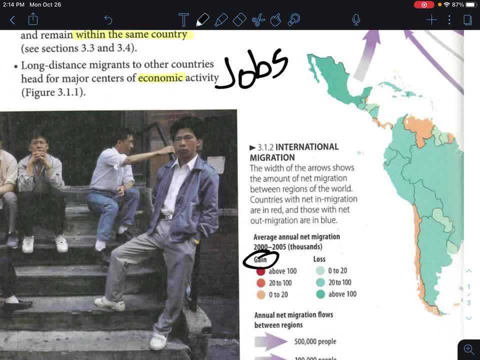 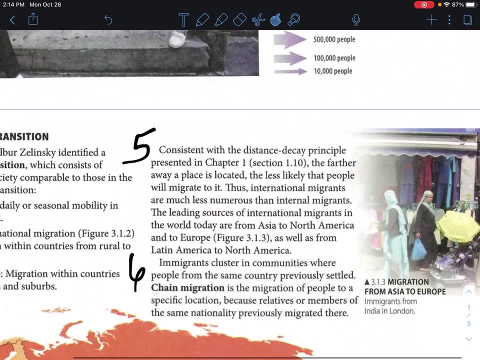 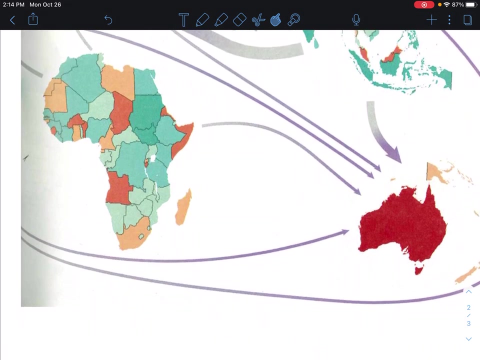 We are gaining migrants And the countries that are in blue with an out migration, they are losing people. So this map here shows us from other regions of the world and it completes that down here. I know it's weird how it splits it, but ideally you would see this on two pages, side by side. You can see. 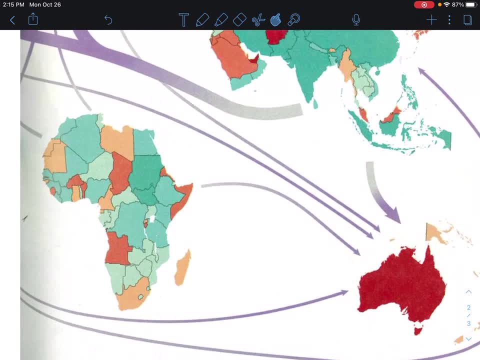 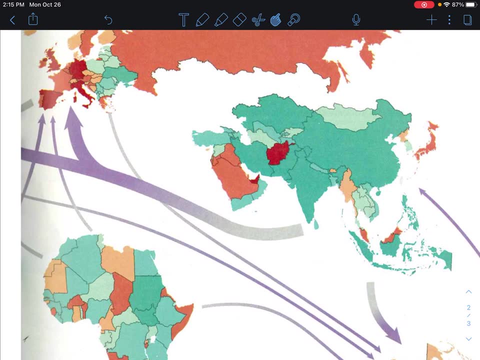 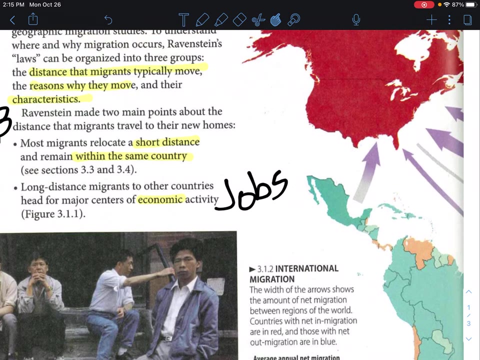 here that Australia gets locked Subtitles by the Amaraorg community of migrants into their country. not too many leaving. you can see here India and South Asia has a large number of people leaving, heading to Europe and heading to the United States. there is a large number of people coming from Mexico up. 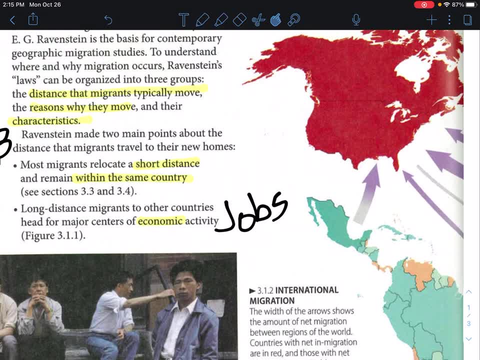 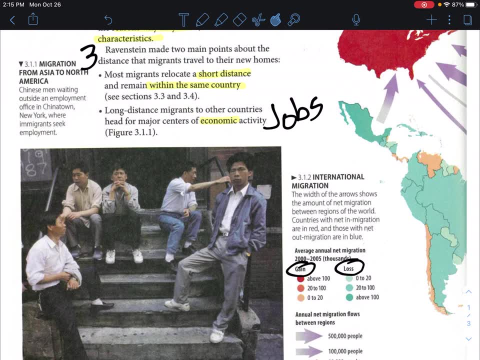 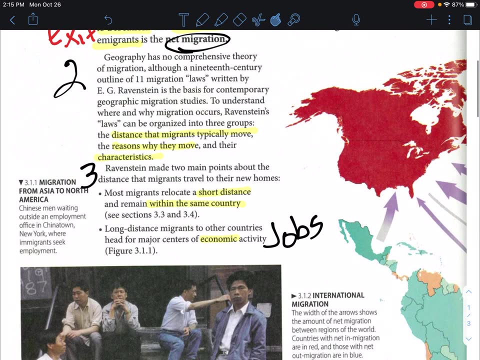 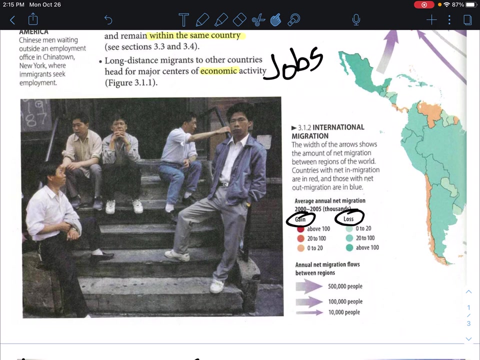 into the United States, maybe Canada as well. so that is three. point one: two: that is showing different migration patterns. also, to look at our numbers, we can see here that United States in Canada is red and they're that deep, deep red. so they have above 100, meaning average annual net migration is above 100,000. but if we 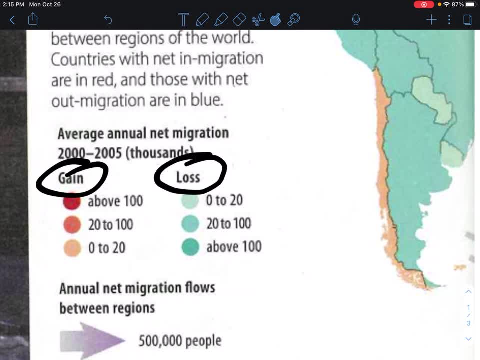 look here, the country along the western coast of South America. this country is called Chile, and Chile has a lower number compared to North America, well, compared to Canada and the United States, but they still are gaining between. well, they got to start somewhere. so between 1,000 and 20,000 people are coming into Chile. now we can. 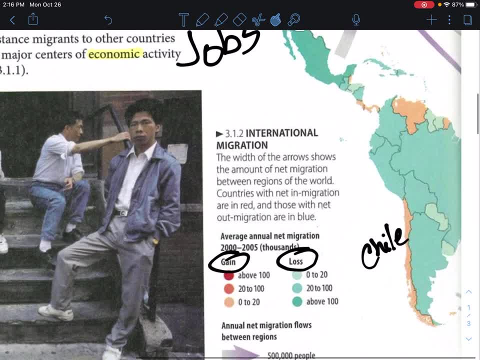 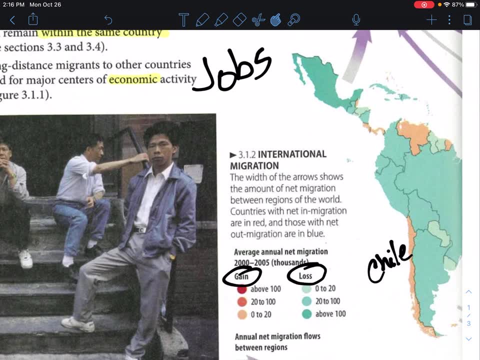 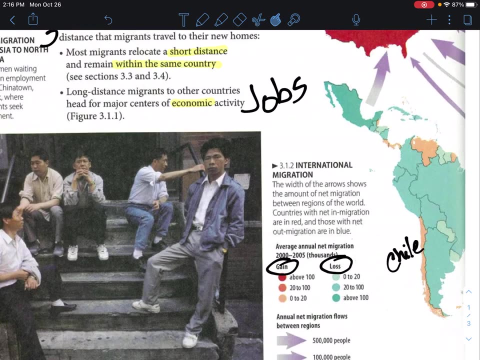 see here that for the most part, a lot of Central and South America are actually losing people from their communities and they're losing people from their countries and that's why they have these different shades of it says blue. it looks kind of bluish green to me, but I think we get what they're coming from. 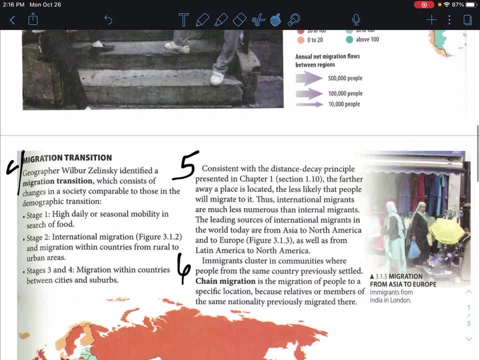 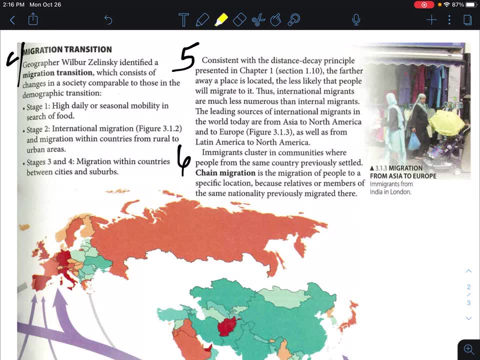 all right, I'm gonna go back to my highlighter and move on to paragraph number four: migration transition. geographer Wilbur Zelinski identified a migration transition which consists of changes in a society comparable to those in the demographic transition stage. one of the migration transition: high daily or seasonal, seasonal mobility in search of food. high 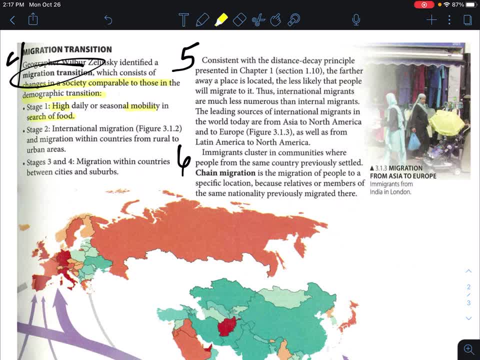 mobility: search of food. stage two: international migration. you can learn more about that from the map. so we just looked at international migration and migration within countries, from rural to urban. so what's another way to say that if I say rural, I usually am thinking about farms and when I say urban, I am thinking about cities. so rural. 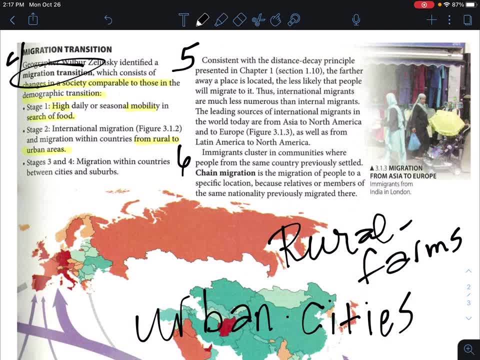 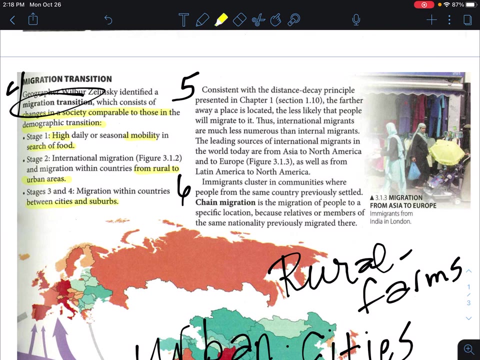 is the countryside and it's where most farming takes place. very agricultural based And urban is in the city and it's more manufacturing and production and service jobs. Let's go back up here. stage three and four: migration within countries, between cities and suburbs. 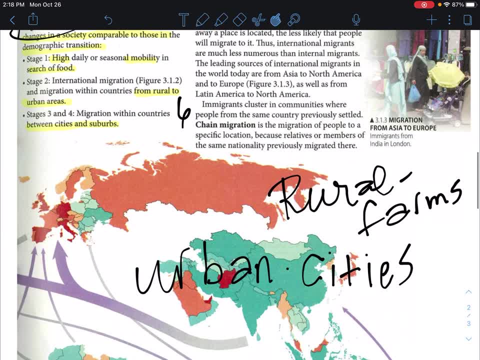 So if we're continuing this conversation, so what is the suburb? A suburb tends to be the- what's a way to say it. If urban is downtown city, this is the outer metro or metropolitan area. So we live in the Twin Cities metropolitan area. 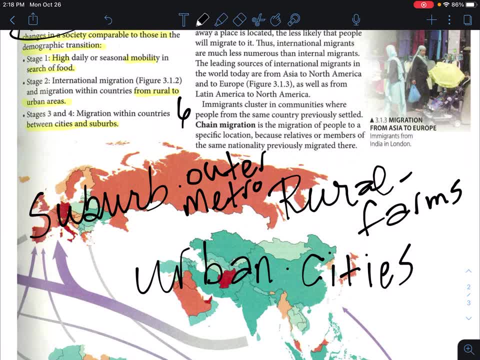 We've got the downtowns of San Francisco, New York and New York. We've got the downtown of St Paul, downtown of Minneapolis. Those are the urban centers And then we start to have the suburban areas: South St Paul, Bloomington, Woodbury, Oakdale. 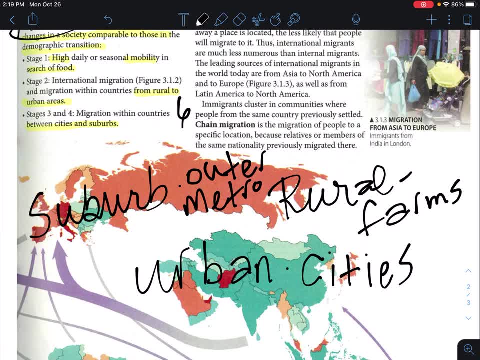 Invergrove Heights, Edina, Minnetonka, Brooklyn Park, Brooklyn Center And up north we've got Fridley and lots of others up there. So the rural is the farmland In between. rural and urban are the suburbs. 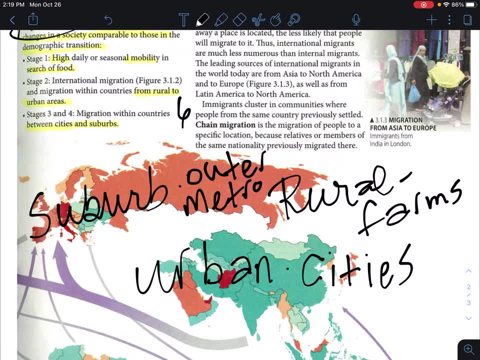 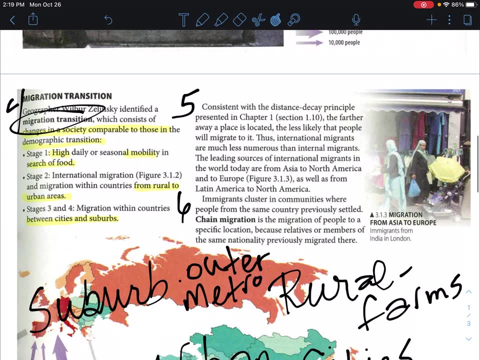 They are the outer metro. That should look like an R there. I'm just going to erase that and put in what looks like an R And then the urban part is the cities or downtown. I'm going to go on to my highlighter with paragraph number five. 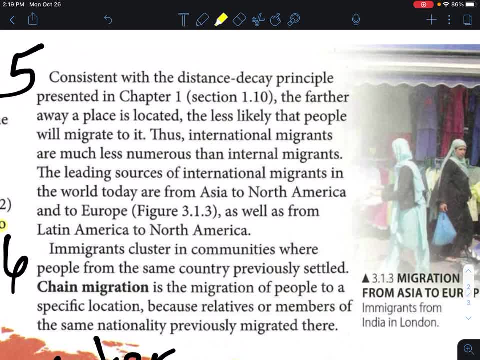 Consistent with the distance decay principle presented in chapter one. the farther away a place is located, the less likely that people immigrate to it. So the farther away a place is, the less likely people will move there. Thus international migrants are much less numerous than internal migrants. 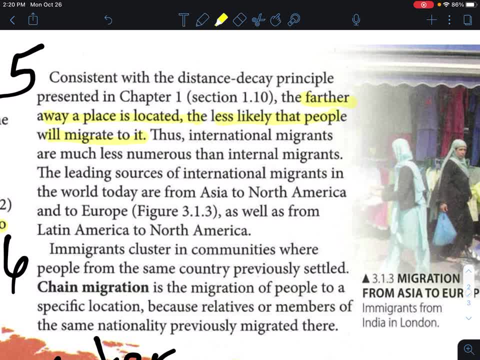 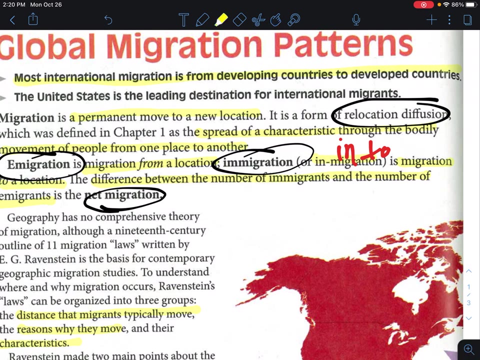 Leading sources of international migrants in the world today are from Asia to North America and to Europe, as well as from Latin America to North America And, as we read a little bit earlier, most here I'm going to scroll up quickly- The United States is the leading destination. 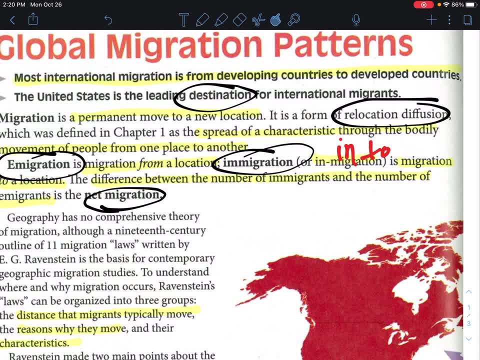 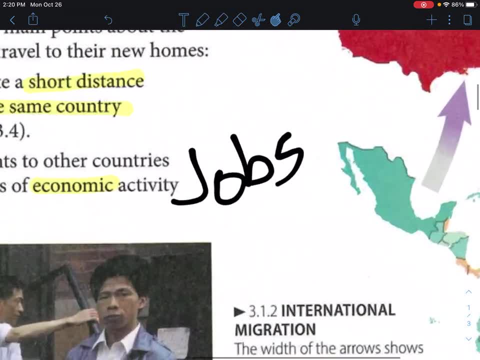 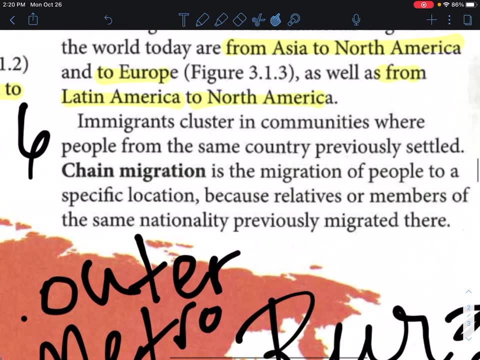 I'm going to circle that word for international migrants, meaning more people are moving to the United States than anywhere else. And why are they coming? They are coming to find jobs. Final paragraph, here is paragraph six. Get my highlighter ready: Immigrant migration. 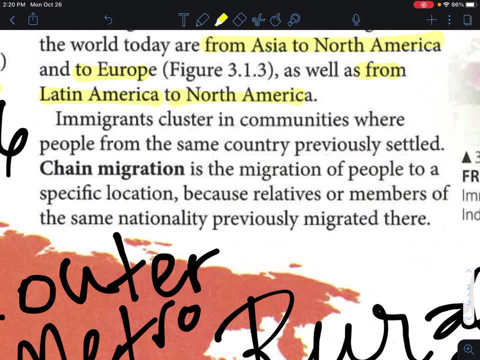 Immigrants cluster in communities where people from the same country previously settled. So these immigrant clusters are usually people from the same country. Chain migration, which is one of our vocab terms, is the migration of a people to a specific location because relatives or members of the same nationality previously migrated there. 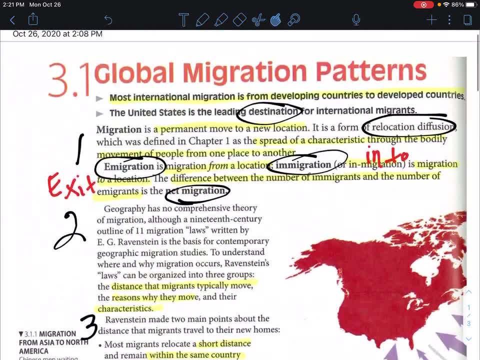 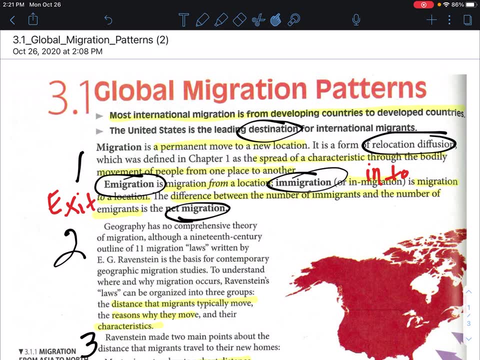 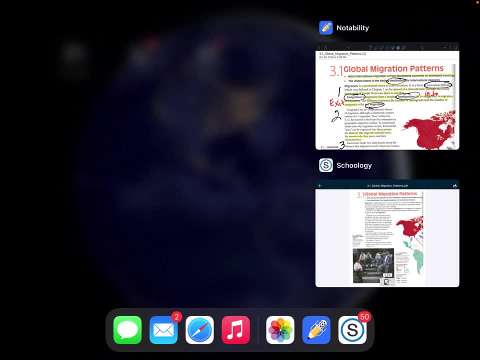 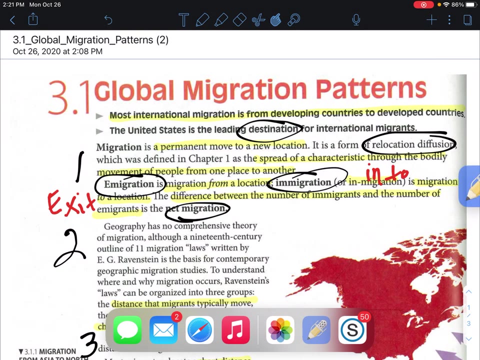 So now that I have read and marked my text, I am going to now open up my vocabulary foursquare. So here's the tricky thing: I don't know how to open two Notability pages at once. I don't think it's going to. let me do that. 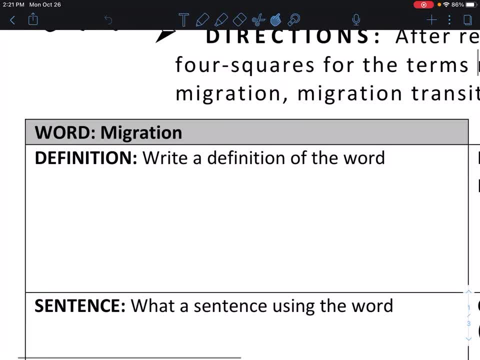 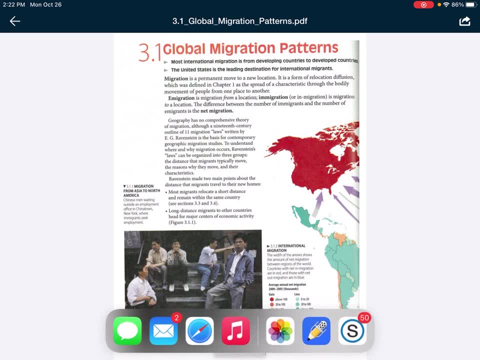 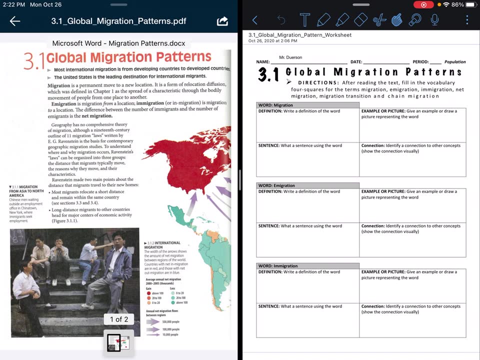 And what I need to do is open up my vocabulary foursquare page, And so, in order to take a look at my reading, I'm just going to have to open up my Schoology reading and have both of these open up at the same time. 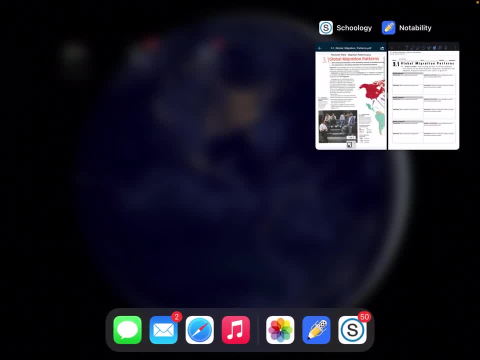 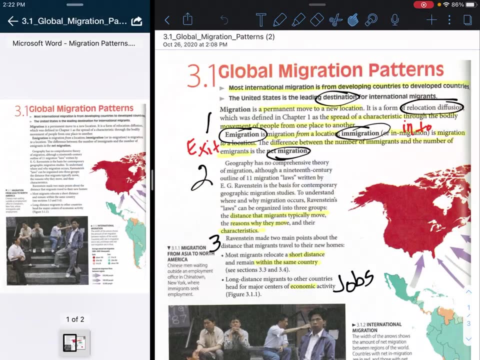 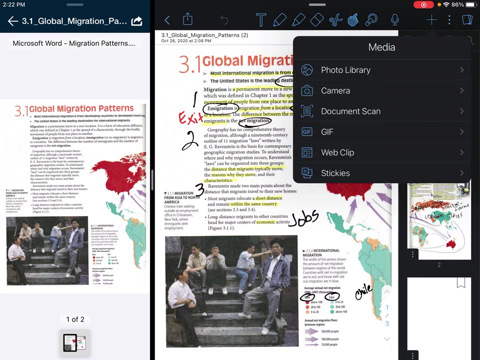 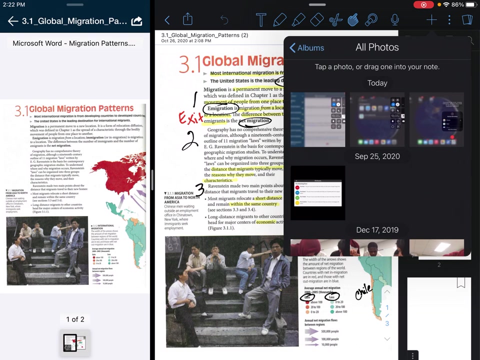 Ideally I'd be able to look at both And I wonder if, when I open Notability, here's my marked text. I wonder if I can actually save that. No, I don't want to do that. I'm not adding it to it. 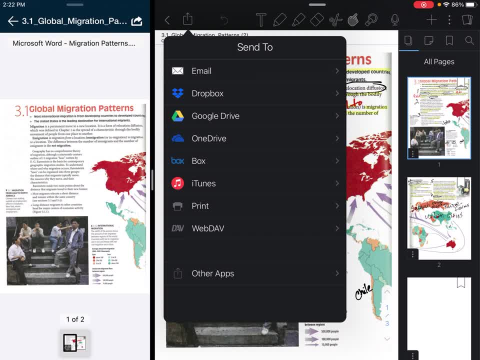 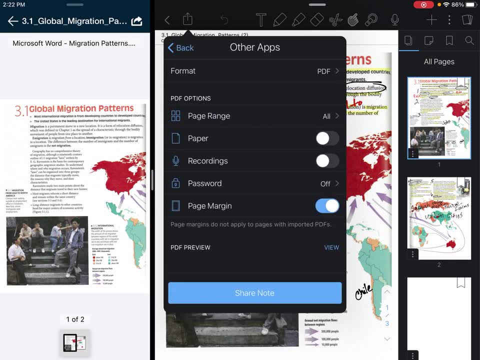 Let's see if I can email it. Nope Other apps. I just want to see if I can open it up and keep it on this page. PDF preview. I do want the PDF and I just want it to sit on my desktop. 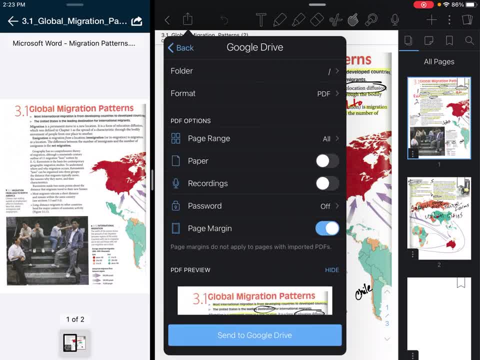 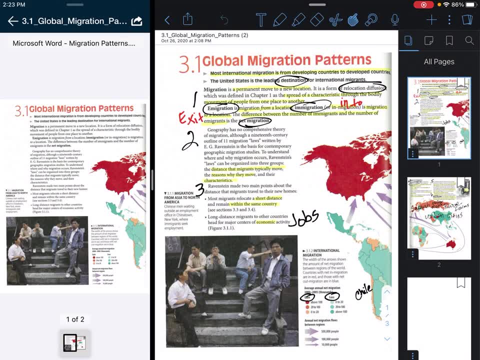 I wonder if I can open it in Google Drive. I don't need a folder, So send to my Google Drive. Nope, Did not send that. Well, I may not be able to view both pages at the same time, So what I'm going to do is go ahead and open up my vocabulary foursquare. 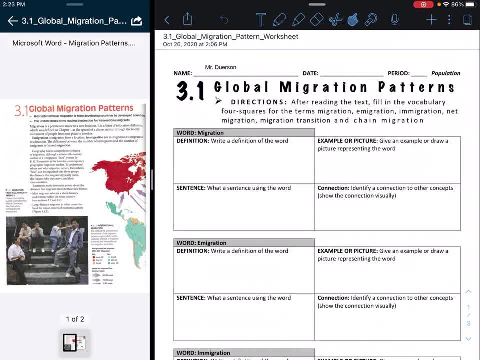 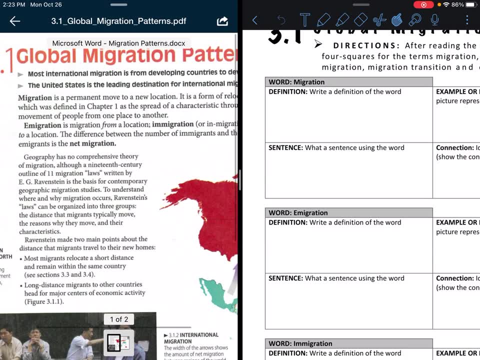 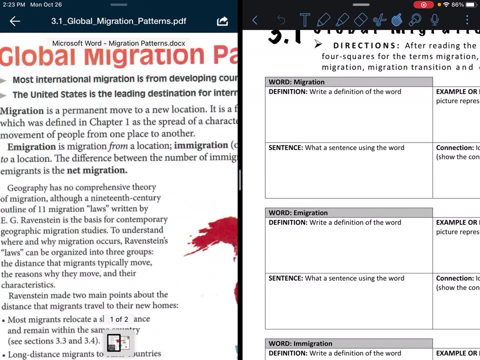 And start filling that part out. My first word that I'm looking for is migration. I need a definition for migration, And I know that migration is a permanent move to a new location. All right, So I'm just going to enter a text box here. 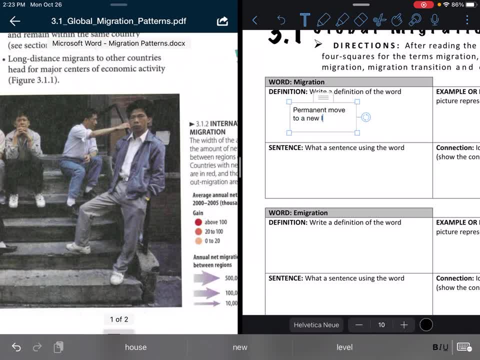 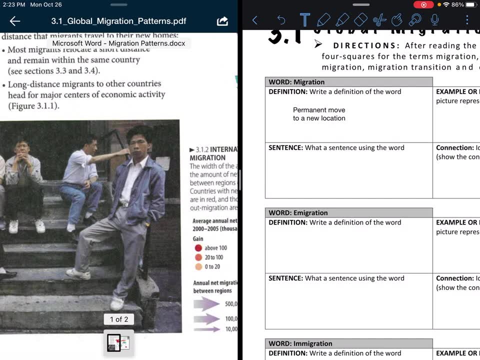 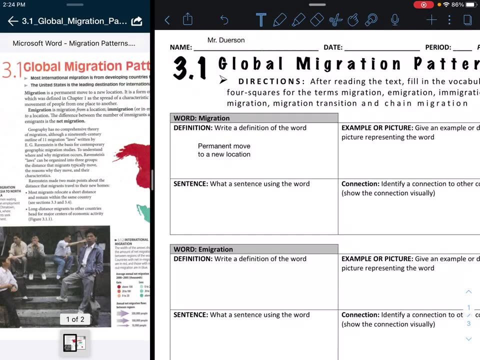 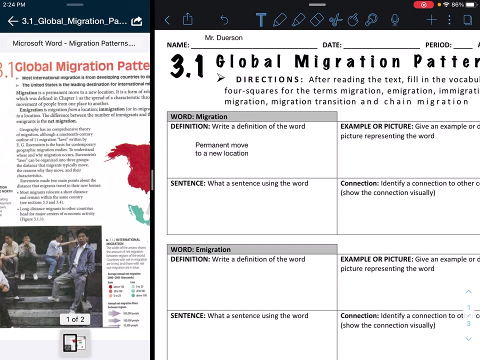 And I'm going to say: a permanent move to a new location And done, I'm done with that, right there. Um, what is a sentence connection example picture I can use for migration? An example sentence: Let's see here. I'm just going to use an example sentence from my reading. 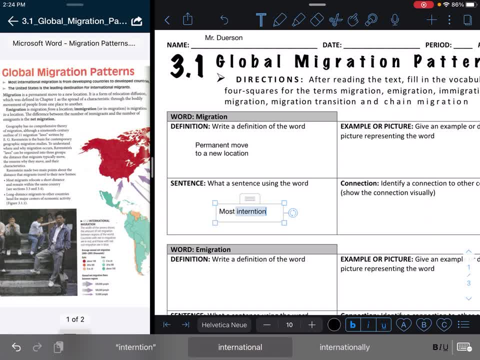 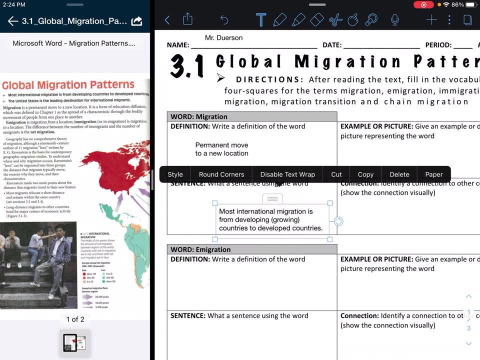 And I'm going to type it in: Most international migration Is from developing. Another word for that is growing countries To developed countries. Now, the United States is still a growing country- More people move here than anywhere else every year- But it's fully developed as far as roads, hospitals, schools, apartment buildings. 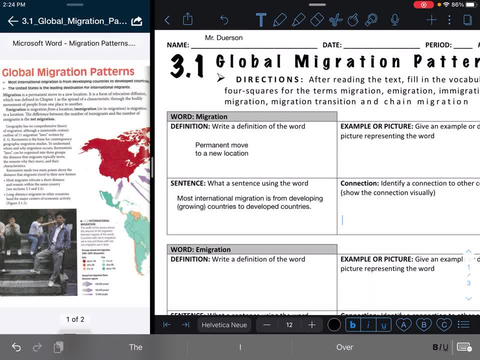 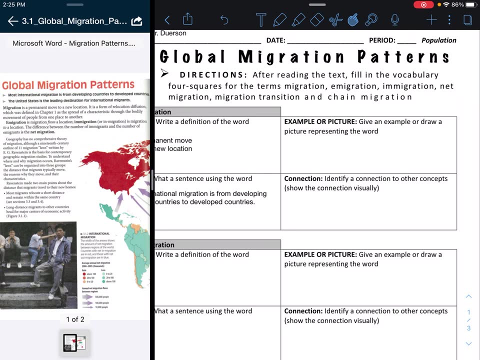 And places to find work. So my sentence is: most international migration Is from developing or growing countries to developed countries. All right, Very good. So I'm going to look at an example, picture and a connection. So connection I'm going to go for next. 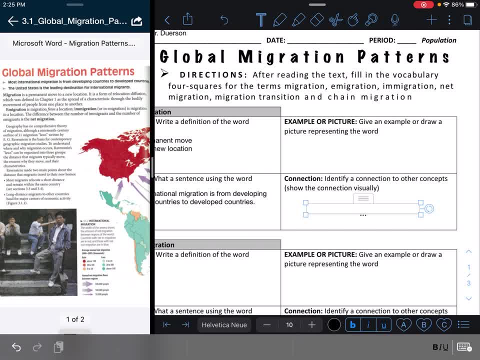 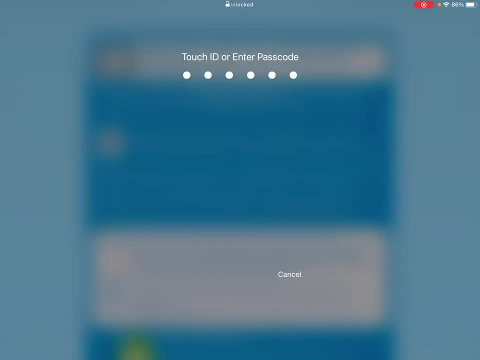 My migration story is something we started our year out with And I'm going to say Mr Duerson migrated From Oklahoma City. Whoops, Oh man, You guys ever like just hit that lock key on accident because it's in a really weird spot. I do From Oklahoma City, Okay, To St Paul, Minnesota, In 2005.. So I've been living in St Paul for 15 years now, So that's part of my migration story right there. I've lived other places in the country. 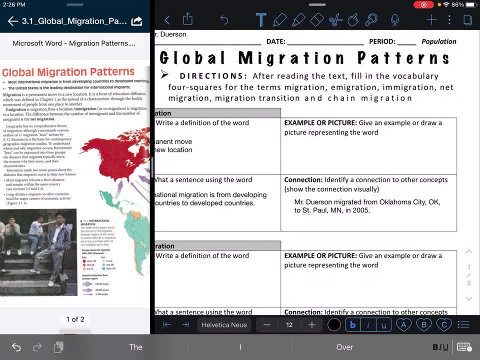 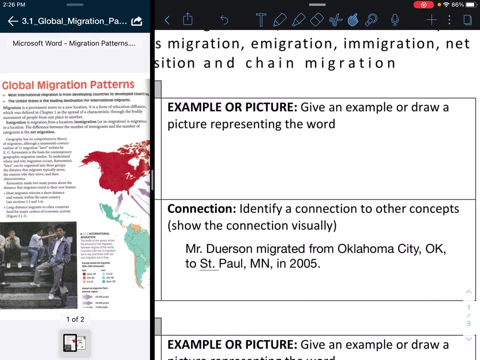 But that is a true statement. I migrated from Oklahoma City, Oklahoma, to St Paul, Minnesota, in 2005.. Now I want an example or a picture. I do find it sometimes very tricky to draw here. Sometimes it's easier to. 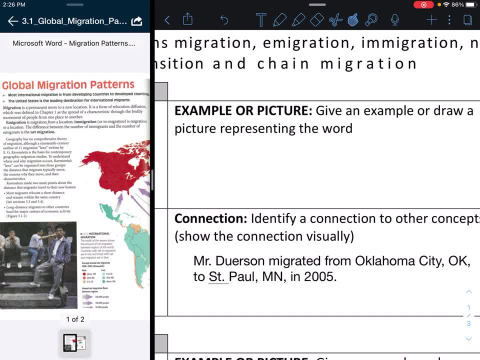 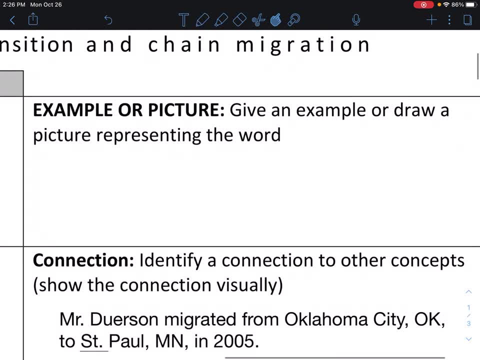 Just find a picture on the internet. Let's see what we can do here. I'm just going to open this fully so I can use this whole page here. So if I do, Whoops, I don't want that, I want a pencil. 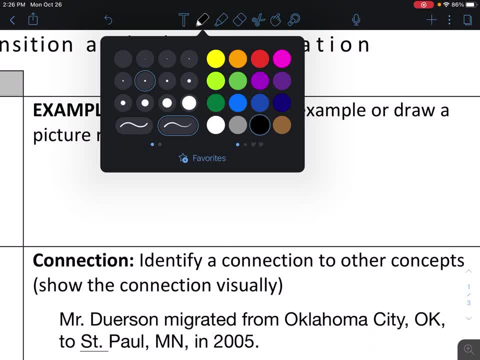 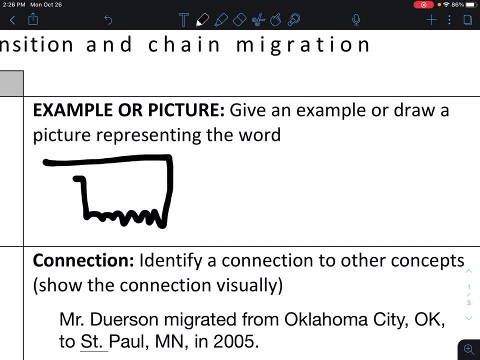 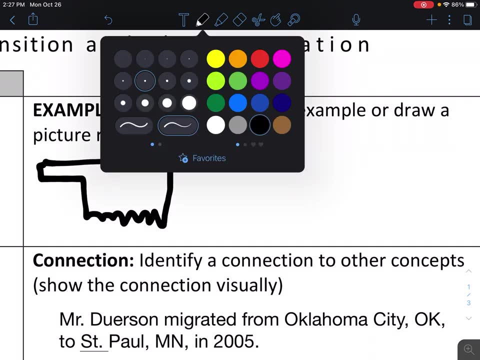 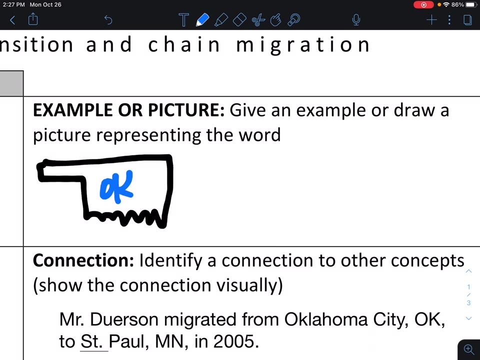 And I want a pencil that's pretty thin. All right, That's good. So I want to draw Oklahoma, That's Oklahoma, And I want a different color, Let's say blue, to represent Okay. And I now want to draw Minnesota. 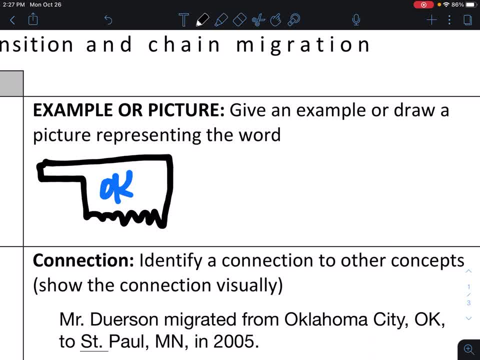 Now, Minnesota is not as easy for me to draw as Oklahoma because I haven't practiced it that much, But let me see what I can do here. Minnesota looks like this Goes over And then we know it does this little thing. Oh whoa. 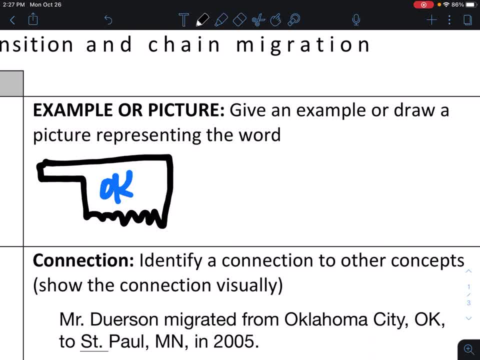 What am I doing here? I'm going to get rid of that. Okay, Minnesota is almost a straight line all the way down, And then it is definitely a straight line across the south, And then it does this sort of curvy thing. 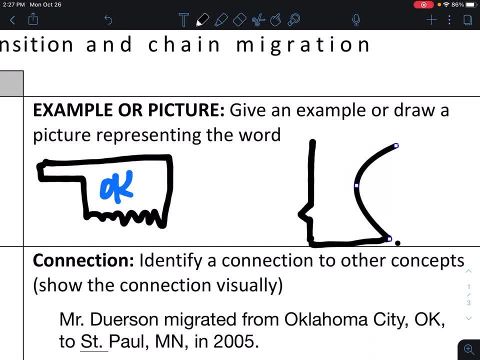 And then it curves back out, And then it Whoops. It keeps thinking I want to move it And I don't. I just I don't want that line though there And I don't want that dot there. Okay, 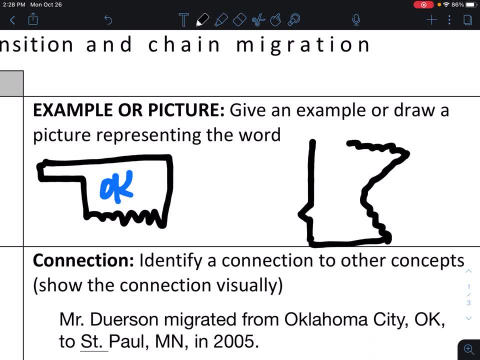 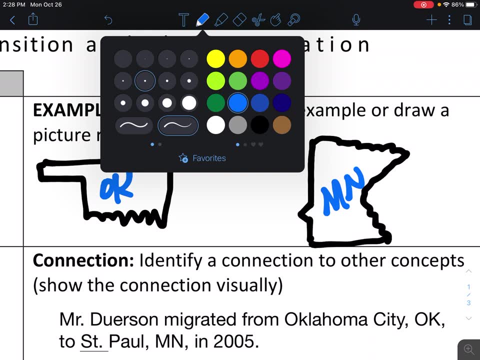 And now I'm just going to connect this. I forgot the little top hat that everybody likes. So this is definitely- though Hopefully you guys will agree- That's Minnesota, And now what I'm going to do is find another color. I'm going to go with green. 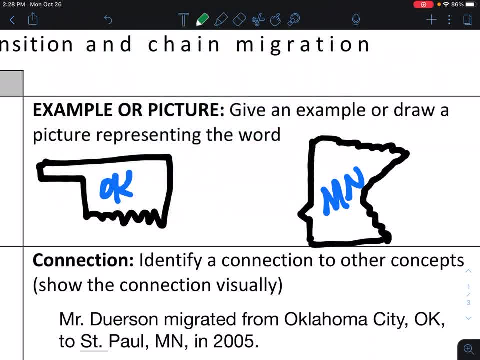 That's my favorite color And that is Mr Dewarson, And I am walking to Oklahoma. I'm going to put a little hat on my head And I am going from Oklahoma to Minnesota, From one capital city to the next. 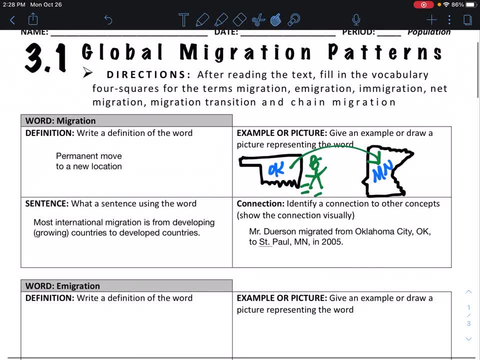 So I have now successfully completed my vocabulary four square for the word four, The word migration. I've got my definition. I have a sentence that I borrowed from the reading. My connection was something that pertains to me personally. I migrated from Oklahoma City to St Paul, Minnesota, in 2005.. 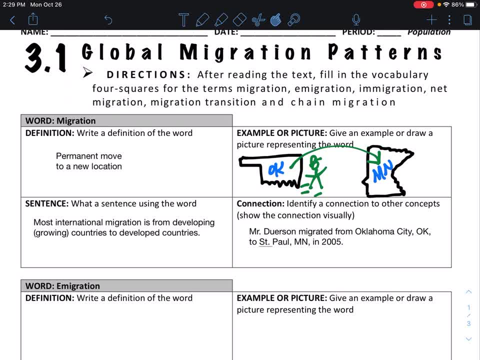 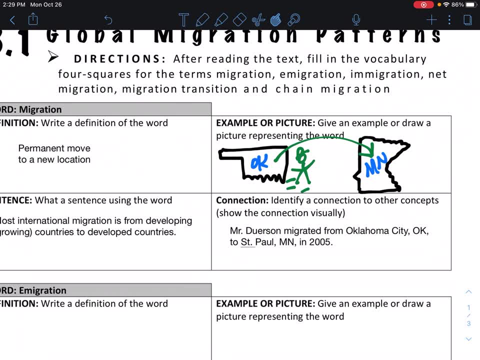 And then I drew a picture of that process- Pretty basic picture, But you know how that works. By the way, if I leave my house in Oklahoma City and drive all the way north to Minnesota, I drive on a highway- Interstate 35- the entire time. 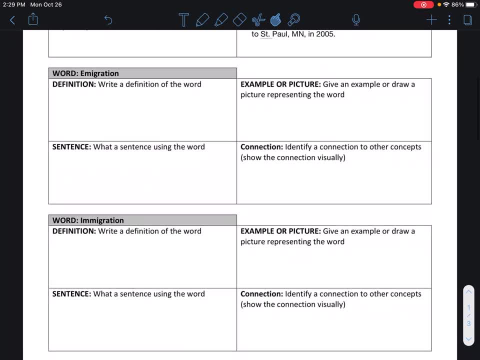 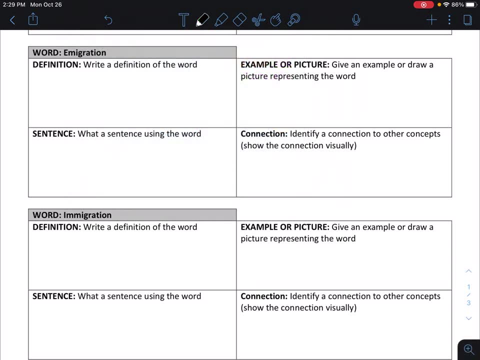 So I now have immigration and immigration. Remember, these are the words that we called homophones, And I'm going to just grab my pencil here again. Immigration. Another word to remember is exit. Let's get that last one off there. 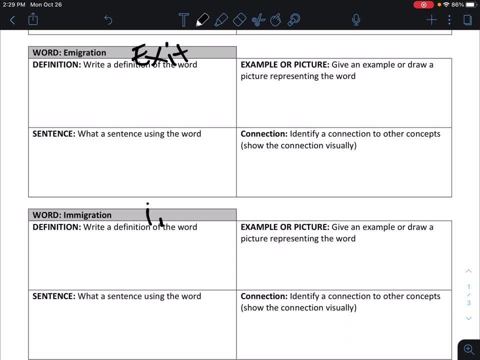 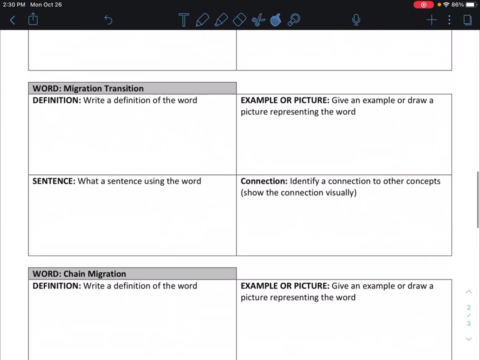 Exit And then immigration with an I is in- That's how I remember it- or in to another country, into can be spelled as one word, but it has a different meaning. So exit for immigration with an E and in two for immigration with an I, and then net migration. 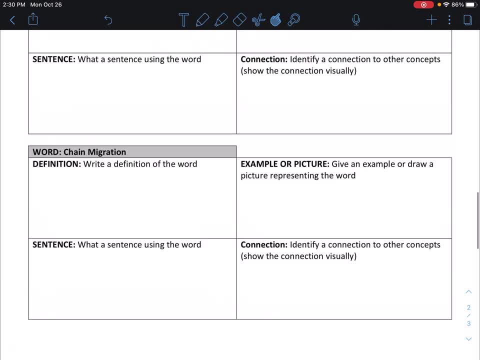 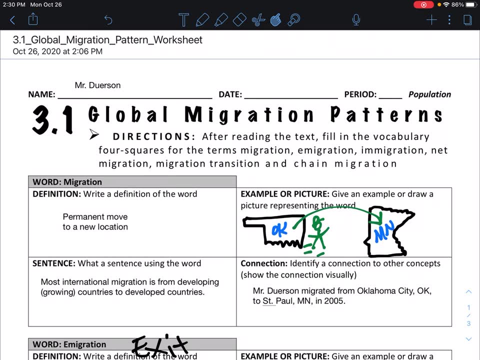 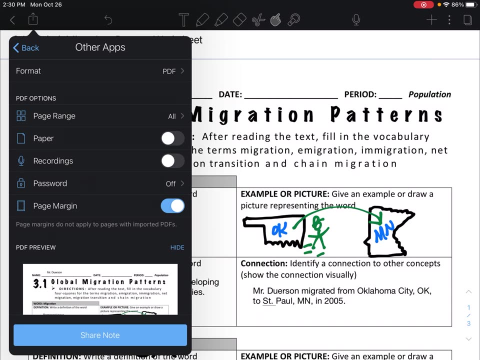 migration, transition chain migration. Spend a little time doing this, but that's why we didn't do any vocab four squares for our ignite. All right, once I'm done with this, you are going to submit this through other apps, and those other apps are going to be Schoology. 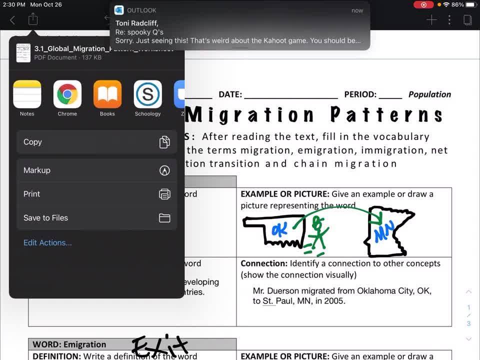 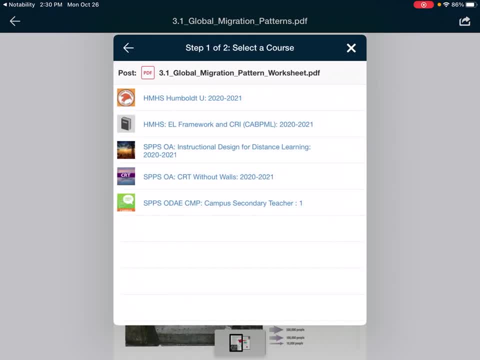 I'm going to share that note and go into Schoology. It's not going to show up the way I do mine or the way you do yours, but I will submit that assignment into 3.2.. I know it's confusing right now. 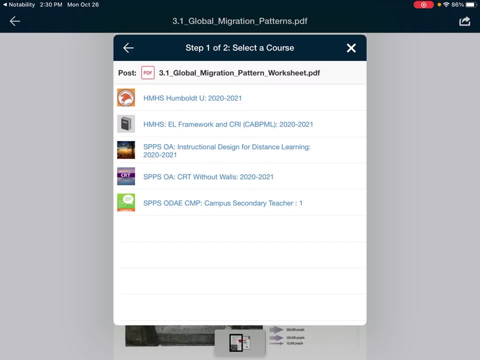 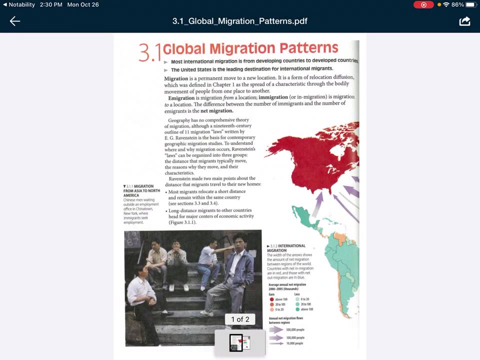 The top of this page is 3.1, but we had to shift it around, So we're definitely looking for 3.2. So I'm going to discard this entry and I'm going to take a look at notability or excuse. 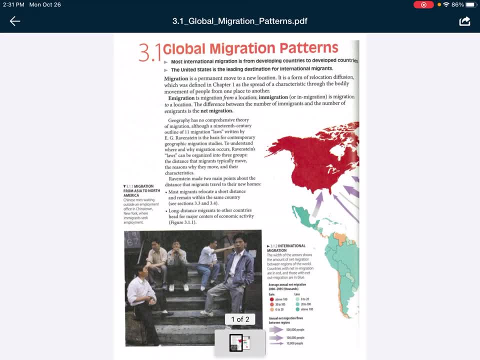 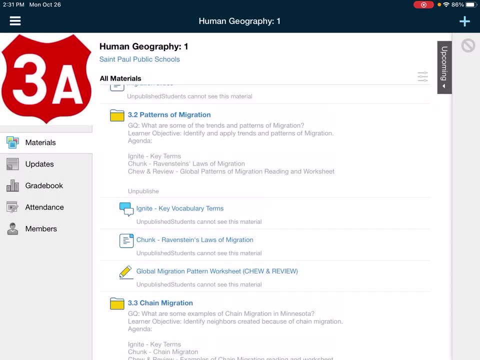 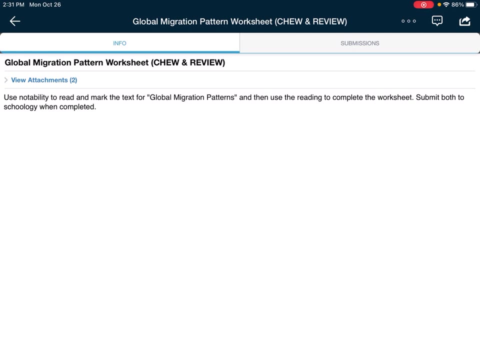 me. I want to look at Schoology. There we go, So it is lesson 3.2 and that's what our global pattern, global migration pattern worksheet- It's going to be under that title: global migration pattern worksheet. Okay, And this is called 3.1..